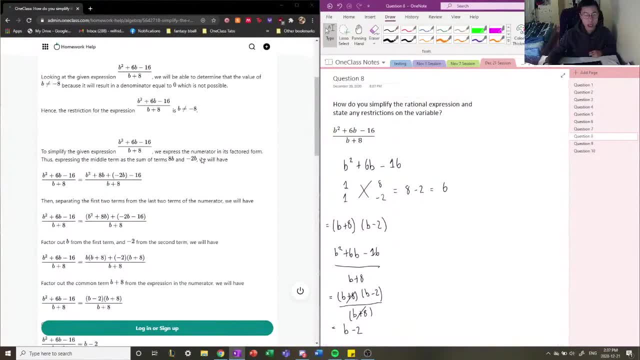 we have to evaluate the original expression, And what they mean by any restrictions on the variable is that for specifically rational expressions and rational functions, there are undefined values, And these undefined values are whenever the denominator is equal to zero, And this has something to do with the limits of a function. We won't get into that in today's lesson. 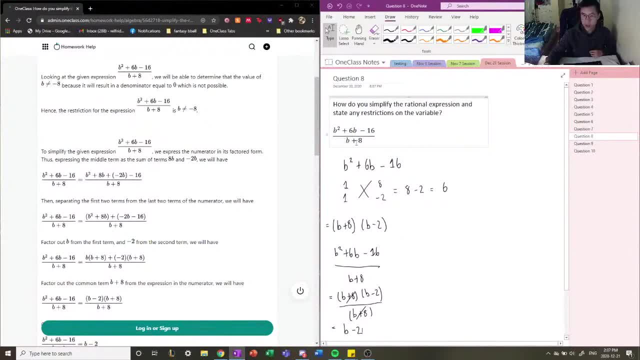 but whenever the denominator is equal to zero, a function will be able to replace it. So whenever a function is equal to zero, a function will be able to replace it. So whenever a function is equal to zero is equal to zero. you cannot divide anything by zero, so we have an undefined value. 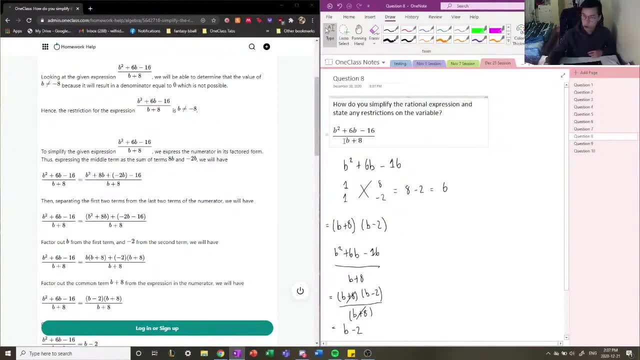 So therefore we have to set a restriction on our function here, or our rational expression, because we do not want to evaluate when the denominator is equal to zero. So in this case, the denominator is equal to zero when b is equal to negative eight, as you can see here. 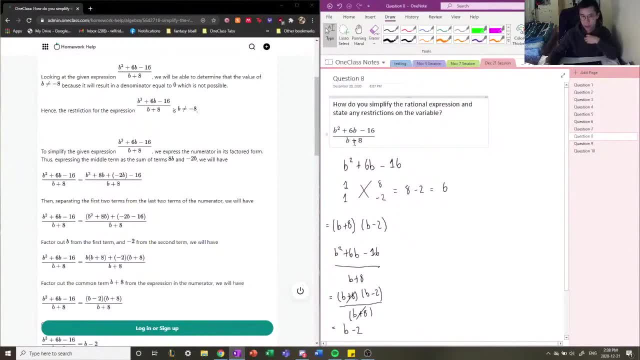 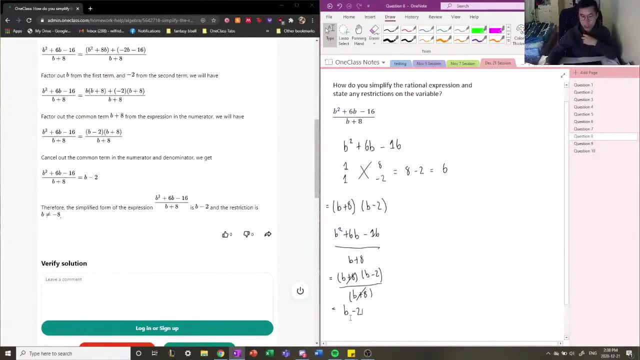 When b equals to negative eight, the denominator is equal to zero, And because of that we have to set a restriction on that. But as we simplify, we see here that when b equals to negative eight, the function is just equal to negative 10.. But when we're setting restrictions on a variable, 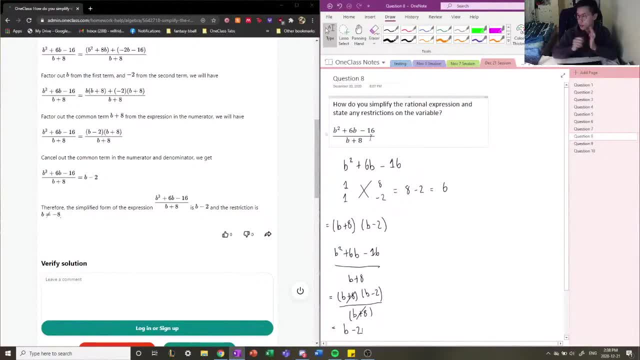 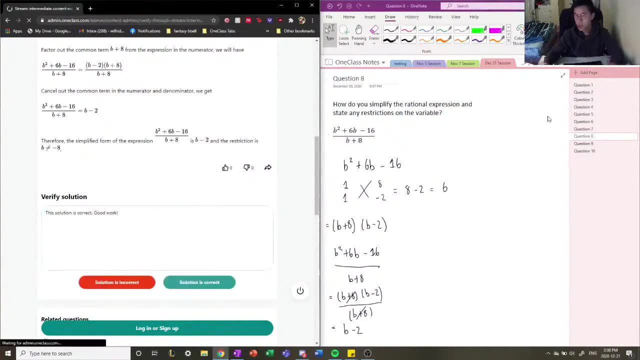 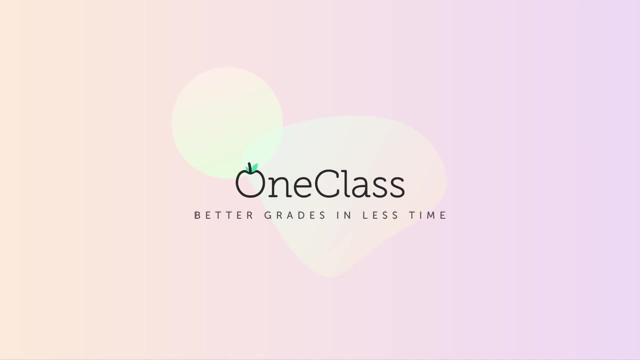 we have to set it on the original expression itself. So the solution is correct. Let's move on to question number nine. Question number nine: 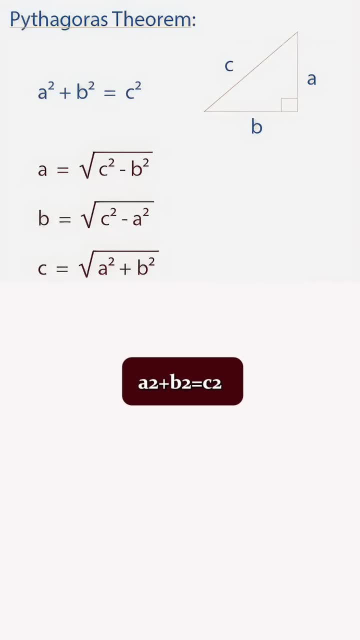 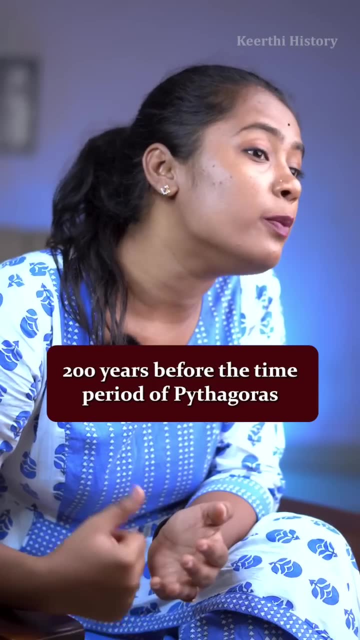 You remember Pythagoras theorem: right A square plus B square equal to C square. What if I tell you that we have mentions of this theory in a book called Baudhyana Salpasutra? 200 years before the time period of Pythagoras, This Indian mathematician, Baudhyana, also wrote: 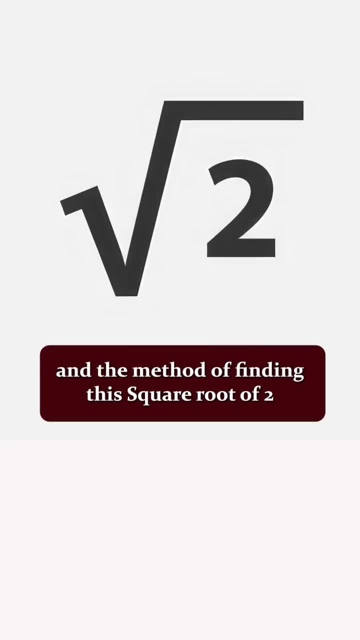 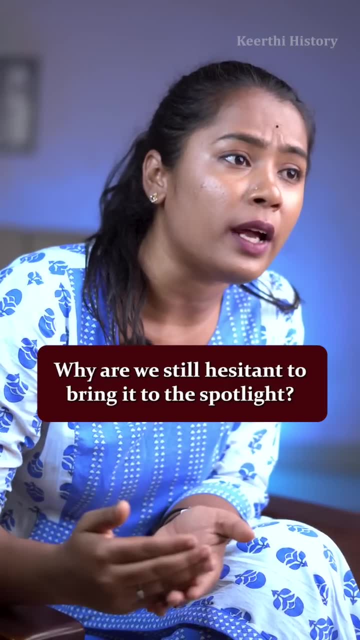 about the value of pi and the method of finding the square root of 2, and many more things. Even though we still have access to all these works, why are we still hesitant to bring it to the spotlight? Leave the rest of the world? At least we Indians should be ready to acknowledge.